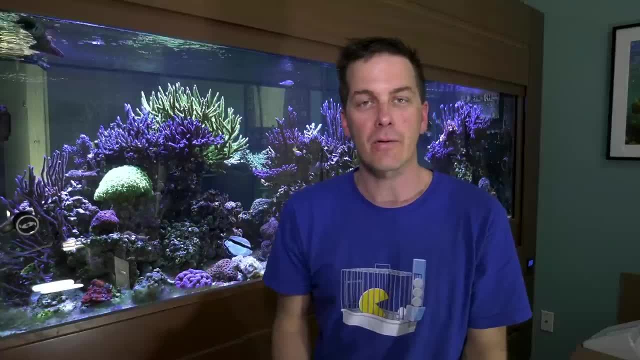 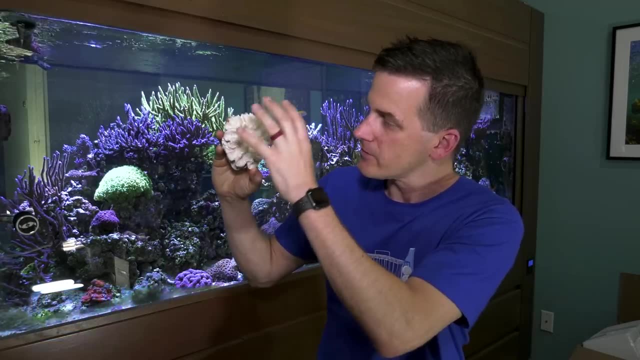 want it growing on other rocks in your tank. 3. Hard Coral. It's called hard coral because they lay down a hard base for themselves, like this one. On this coral skeleton you still have coral polyps, and as the polyps grew, they laid. 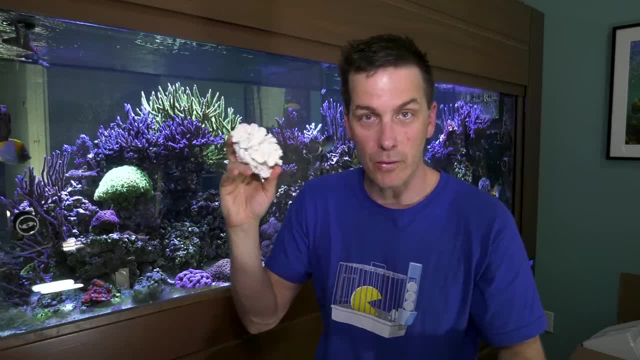 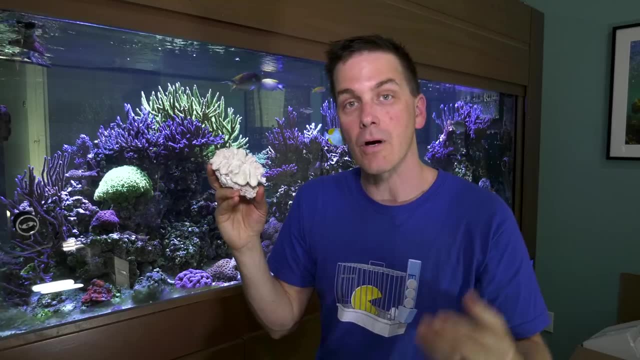 down calcium carbonate to make this skeleton, hence the name hard corals. Corals need certain things out of your tanks water to build this twist system around our Because don't come to build this calcium carbonate skeleton which, as a general rule, hard corals have more intense. 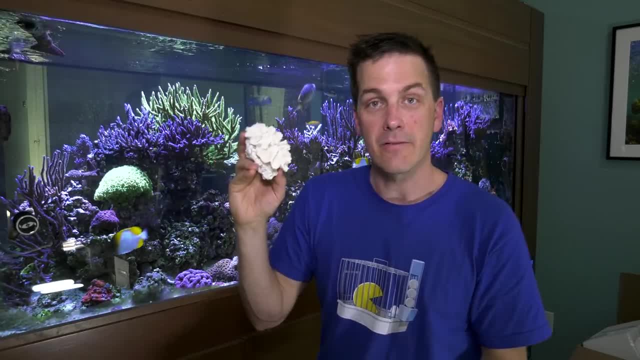 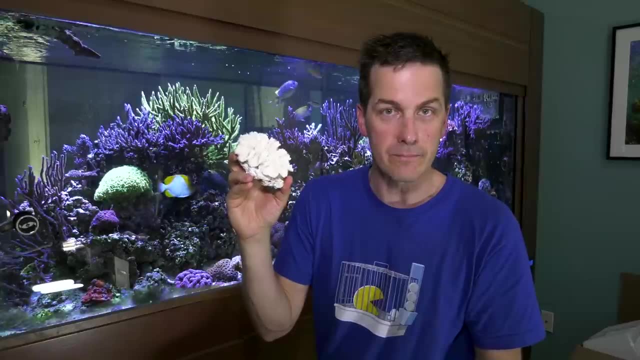 needs than soft corals. I'm going to talk about those needs in a minute. For now, know that if you're looking at a coral and it has a hard base like this, you can see some kind of skeleton structure. you're looking at a hard coral. Hard corals can be broken down into two categories. 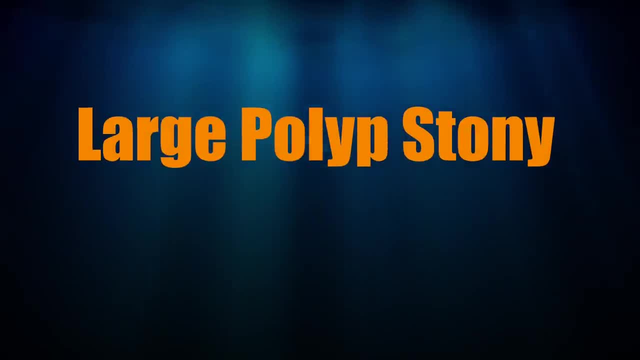 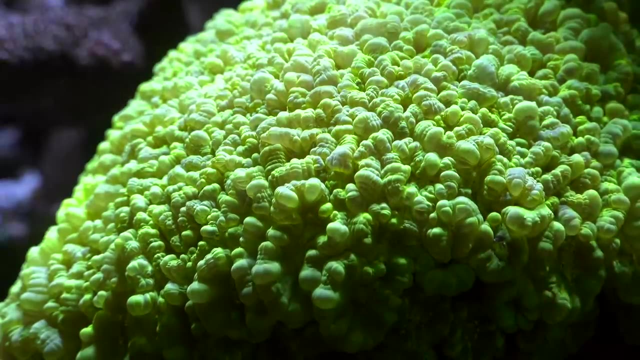 LPS, SPS. LPS stands for large polyp, stony coral, Large polyp, as the individual polyps are well large. Here's an LPS coral in my tank and each of these guys is a polyp. 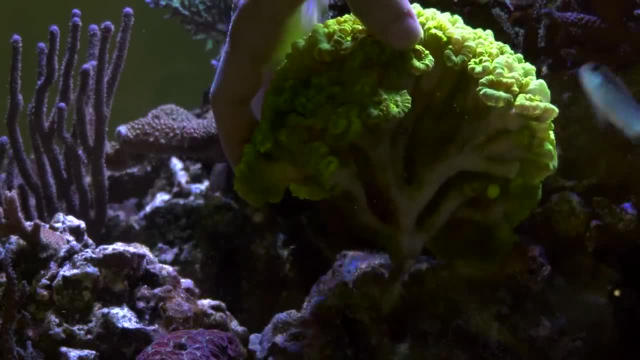 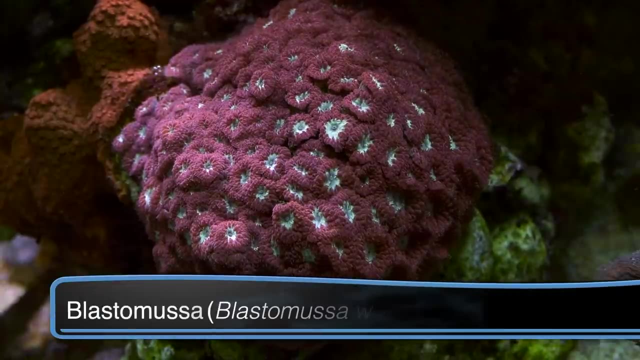 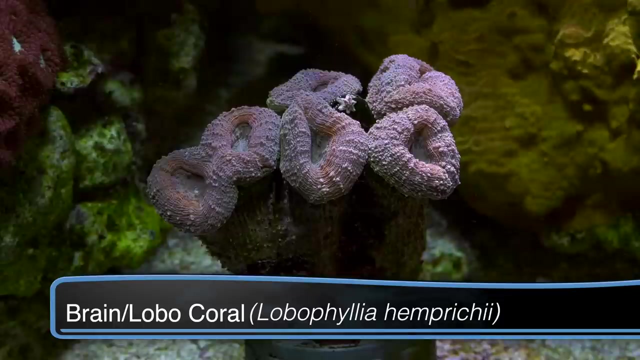 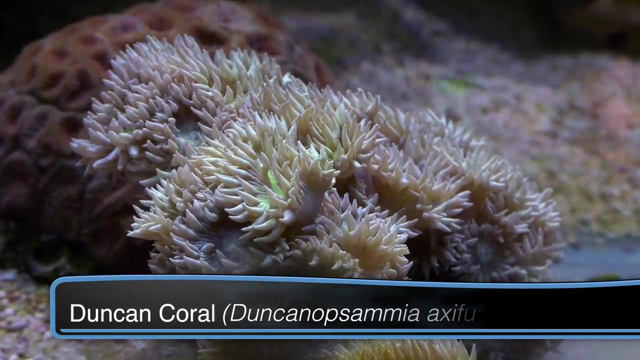 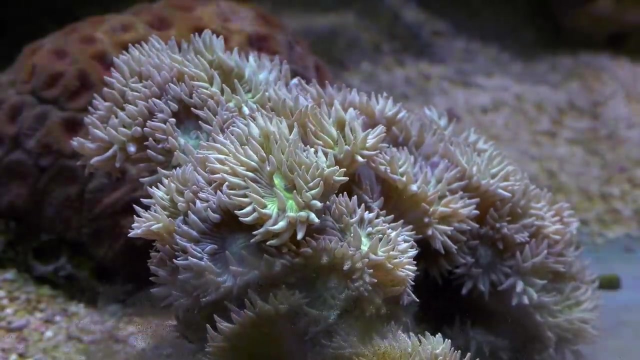 Underneath all that flesh is a hard skeleton, which is why it's called a stony coral. Here are other examples of LPS corals. Contrast this LPS coral with this SPS or small polyp stony coral. The SPS coral has small polyps. 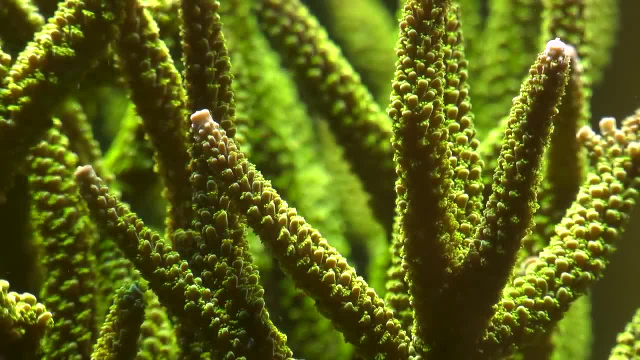 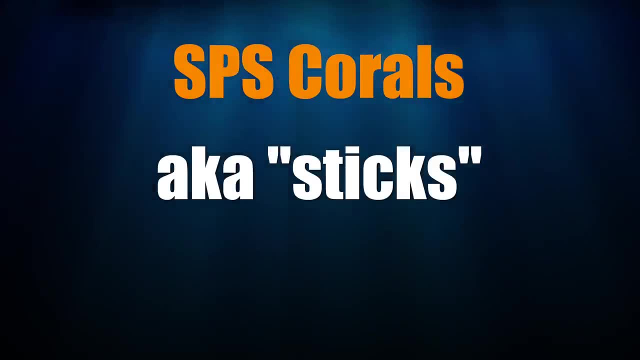 Sometimes they're so small you can hardly see them. Underneath all that color is still a hard skeleton, Affectionately referred to as sticks by reefers. SPS are easily fragged and traded or sold. They come in all different shapes and colors to create a splash of color in your reef tank. 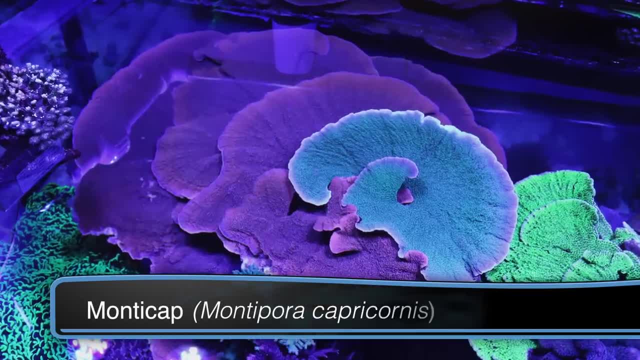 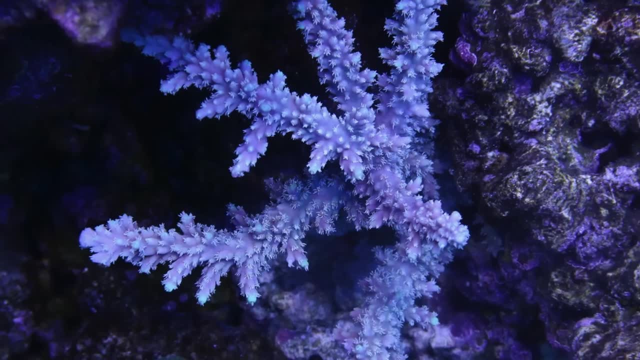 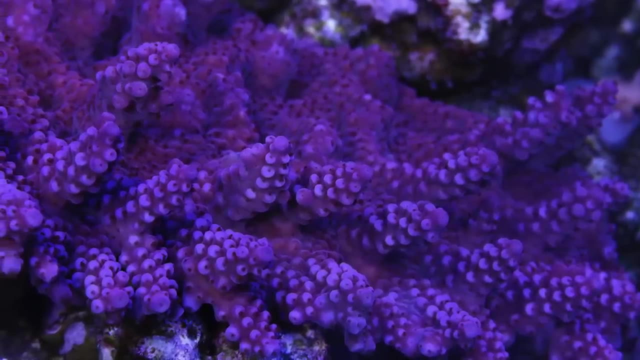 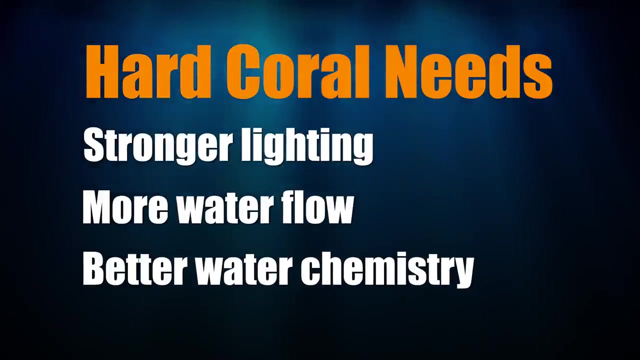 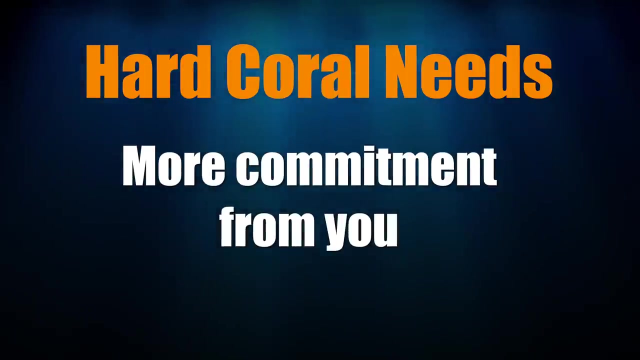 A general rule of thumb for hard corals is that they need stronger lighting, more water flow inside your tank and better water chemistry. That means more gear and time on your part. That doesn't mean a lot of time and a lot of money, and part of the series is me walking.